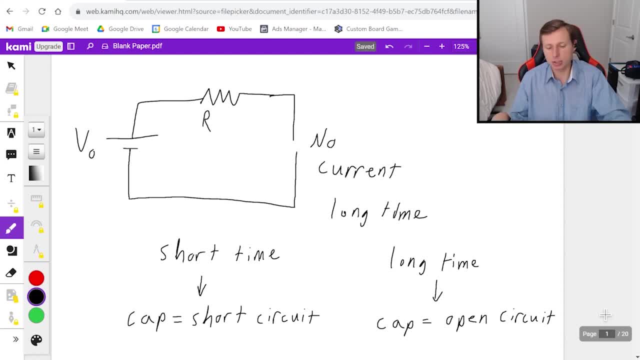 current through. The reason why it does that is because we say the capacitor is fully charged. I want you to think of the capacitor like a bank for charge And once the bank is full it can't let anyone else in. So maybe like a nightclub is a better example At first. 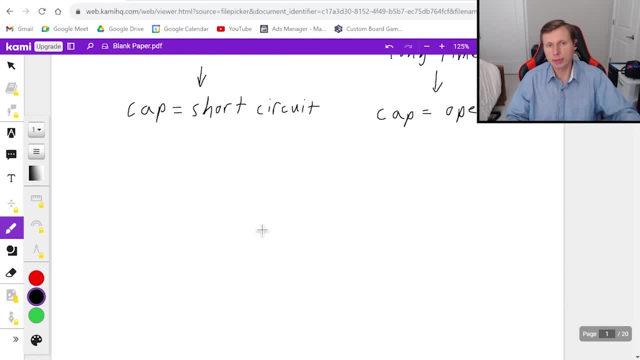 you got to let people in, then you're full. then you say no more. Now let's talk about the equations associated with the RC circuit. We say that when the RC circuit is charging. that's the exact situation I just laid out a minute ago, the voltage in the capacitor, which let me just draw. 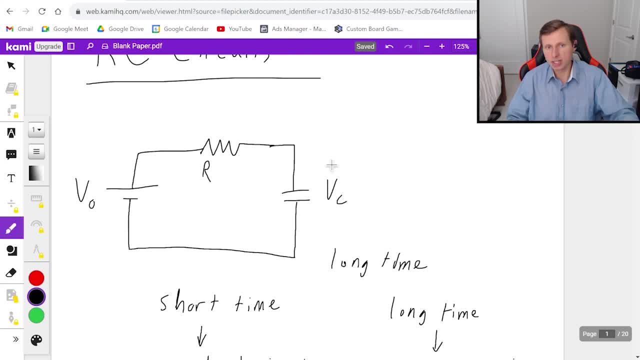 that real quick. We're saying the voltage in the capacitor VC, positive, negative. if you were to actually measure this voltage, then the voltage would be equal to V, naught times the quantity one minus E. to the negative T over tau. I don't know if you have to have this equation memorized. 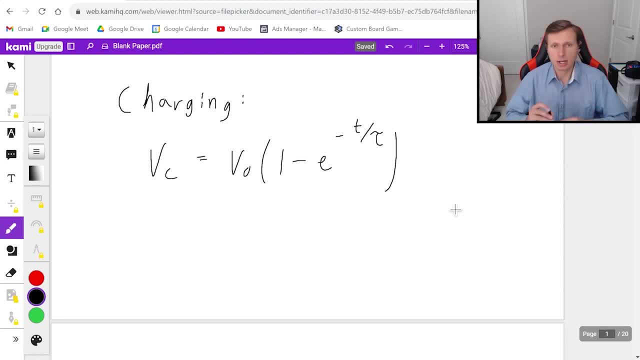 or not. It could be on your equation sheet, in which case you don't have to. Having said that, I would have it memorized because I had to, but that's because I was an electrical engineering major, And hopefully you're smart enough not to be an electrical engineering major. 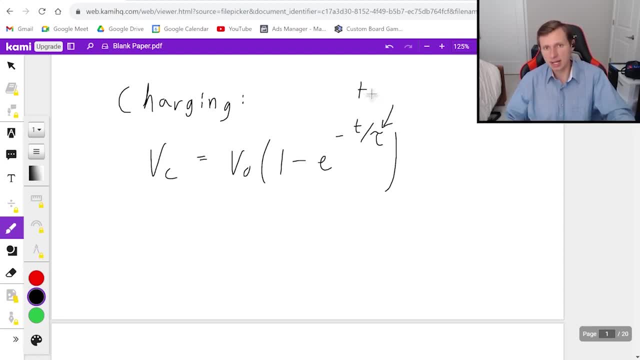 Also this tau right here that's known as the time constant And basically what the time constant is is. it describes how quick or how slow the response is to this charging capacitor, And I'll explain that more in the graph that I'm about to draw. 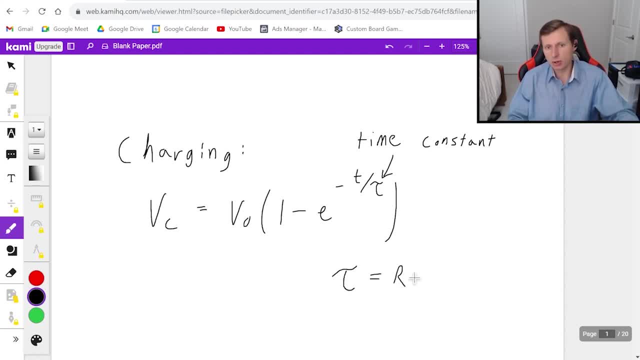 in a minute. But first tau has an equation. It's equal to R times C, the resistance times the capacitance. And if I wanted to draw a graph of this voltage over time, here's the voltage in the capacitor, here's time. So at the beginning there's no voltage at all. That's because of the. 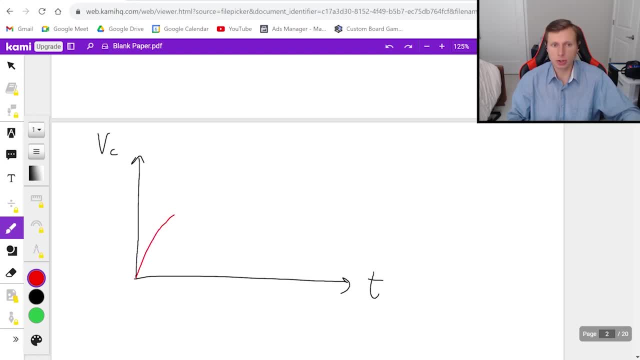 voltage in the capacitor. So at the beginning there's no voltage at all. That's because of the short circuit aspect. But it's quickly going to charge, charge, charge, charge, charge. And then, once it gets close to being full, there is a horizontal asymptote in this graph where it cannot. 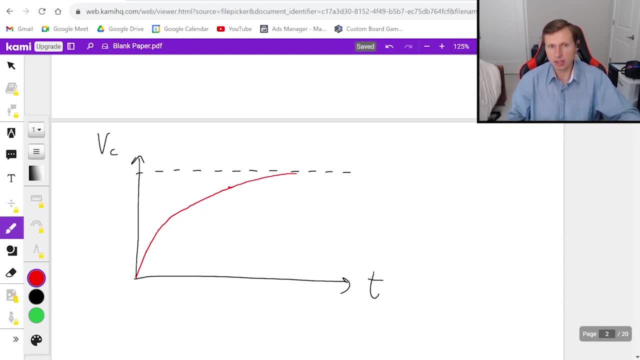 actually ever touch this number, but it can get very, very close. So it's essentially touching it And that limit, that highest value is V9.. It's the voltage on the battery which makes sense. And just to show you what the graph would look like with a smaller time constant, it would look like: 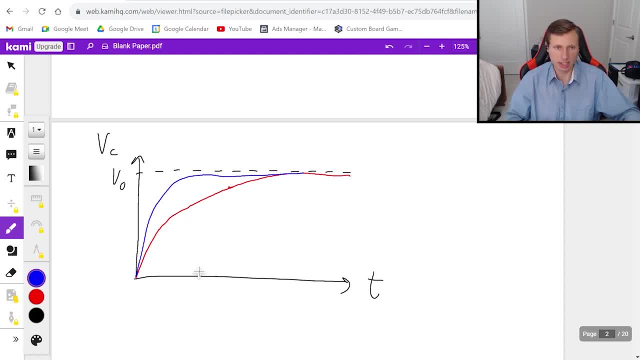 this And just to show you what the graph would look like with a smaller time constant. it would look like this: In other words, it gets charged very, very, very quickly. So the blue is for a low time constant tau and the red is for a high time constant tau. A low time constant means it. 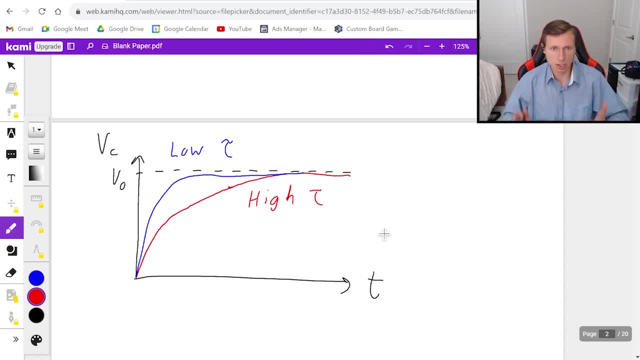 charges quickly. A high time constant means it charges slowly. And then one last thing I'll say about this is that we can also measure the voltage in the resistor. The voltage in the resistor is just going to be the voltage in the battery, minus whatever the voltage in the capacitor is. And 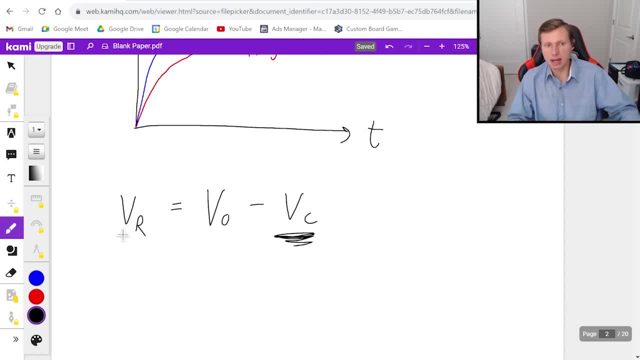 obviously the voltage in the capacitor is just going to be the voltage in the capacitor And since this value is changing constantly, that means the resistor value is changing constantly. As a matter of fact, we would say at first the voltage in the capacitor is zero. 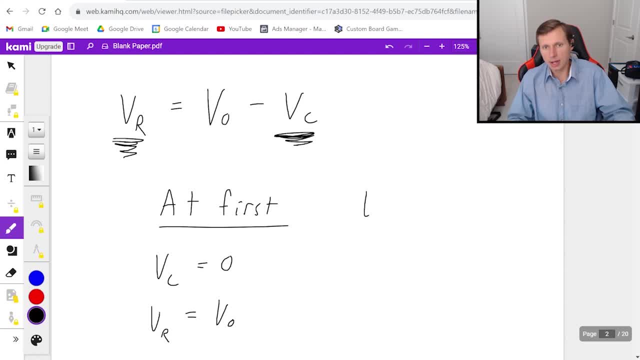 which means all the voltage is in the resistor. But after a long time, like we said, what happens with this RC circuit? the capacitor then becomes fully charged VO and the voltage in the resistor is zero, And that has to do with the fact that we're not getting any more current. 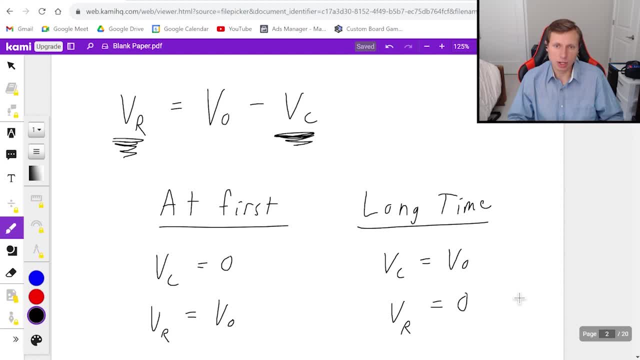 So that's basically everything you need to know for the charging scenario. Now there's one more thing that can happen here. It's possible that you can have a switch in this RC circuit. So in other words, I'm just adding a switch right here at the start. Initially maybe it was. 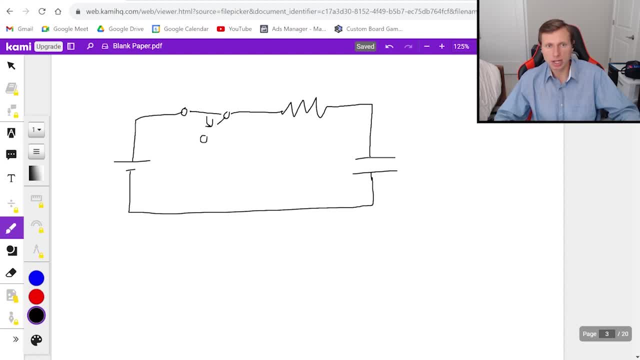 connected like this, but after a while maybe we flipped the switch and now the circuit is connected here And when you move the switch to this position, you can see that the circuit is connected here And when you move the switch to this position, what you need to know is that you. 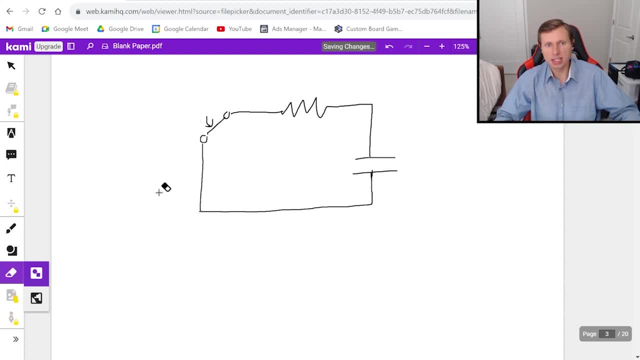 essentially just cut off the battery entirely, and now you're just left with this little circuit that is literally just a capacitor and a resistor. When this happens, even though there's no battery, the current is still going to be flowing. You'll still have a current at least. 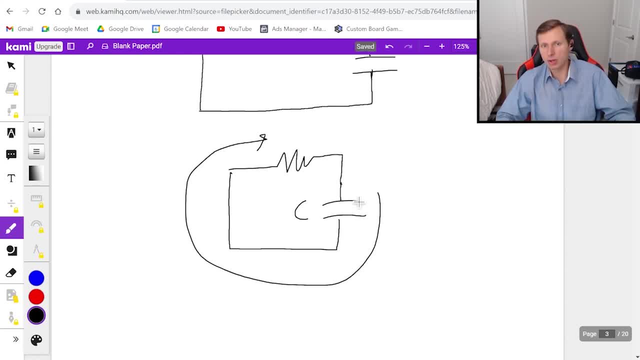 for a short time. The reason why is because your capacitor still had all that charge stored in its bank. but, very quickly, the electrons are going to leave the capacitor and then, after a long time, everything's going to be zero, VC is going to be zero. 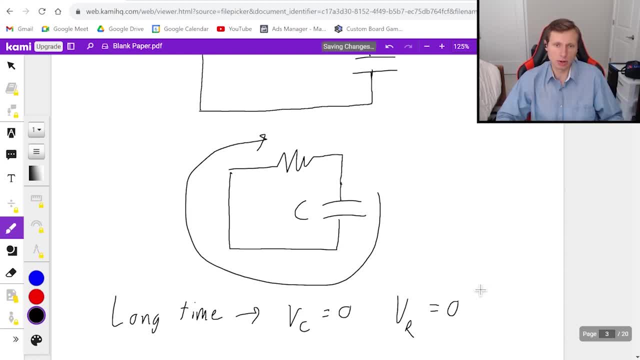 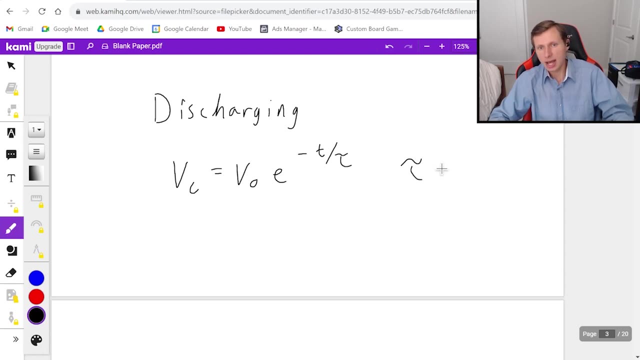 and VR is going to be zero because you've run out of charge, like having a battery that ran out of power. So then the discharging equation is very similar. It's going to be: VC equals V naught times E to the negative T over tau. or again, tau is equal to R times C. Look how similar that is to. 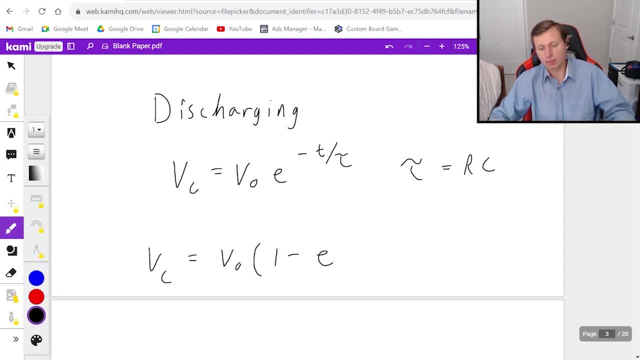 the charging equation. The only difference is that when you plug in the battery, the current is going. difference is the one minus in the parentheses. This is the charging. Above is the discharging. Very similar equations, but they work opposites of each other. So, in other words, if I were to 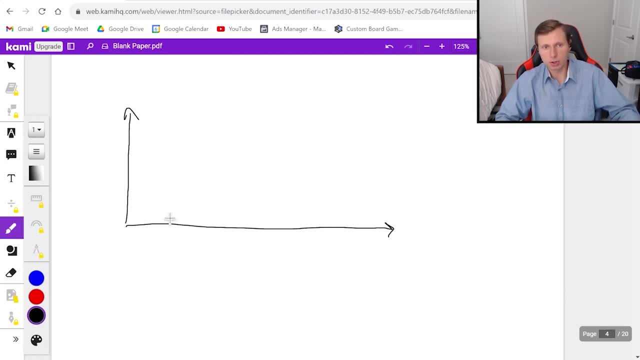 continue that graph that I was making before of the charging versus discharging capacitor, where let's say, here is my V, naught my peak voltage. then, when we're charging, the graph looks like this: And then let's say, at this point, right here, we flip the switch and all of a sudden, 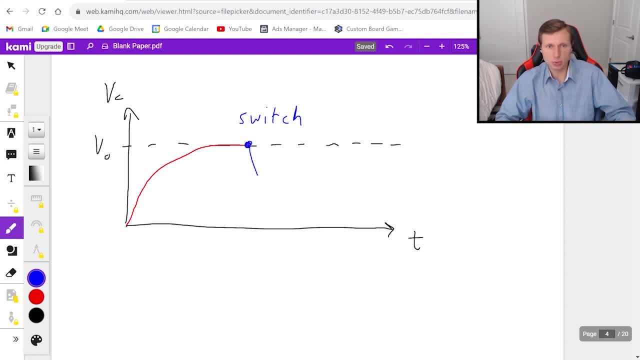 we start discharging. Discharging looks like this: We shoot downwards and then we trickle, trickle, trickle until we get to zero. And then, let's say, you hit the switch again right here, which is totally possible- Then you're going to have charging again. So the red is a charging. 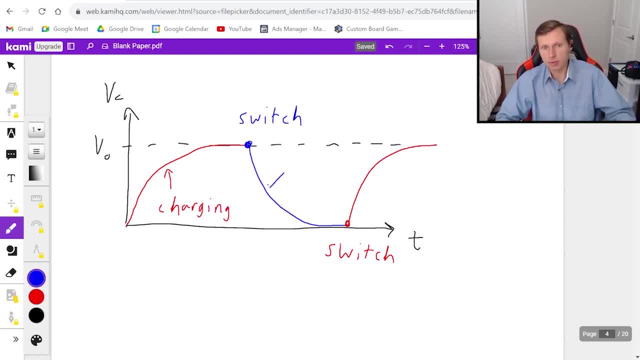 capacitor. It's the graph for a charging capacitor And wherever you see blue, that's the discharge And that's basically everything you need to know for RC circuits. So definitely study all of that. Make sure you've become familiar with the charging versus the discharging, the open circuit versus 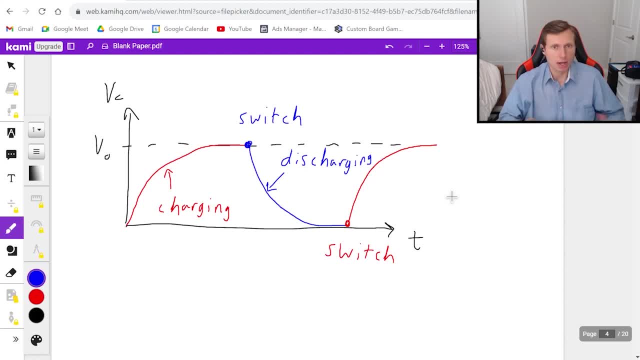 the closed circuit, how the capacitor and the resistor behave after a short time and for a long time, because all that stuff can show up on the test. So thank you all for watching. I hope you have a great rest of your day and I'll see you in the next video. Take care and bye-bye.